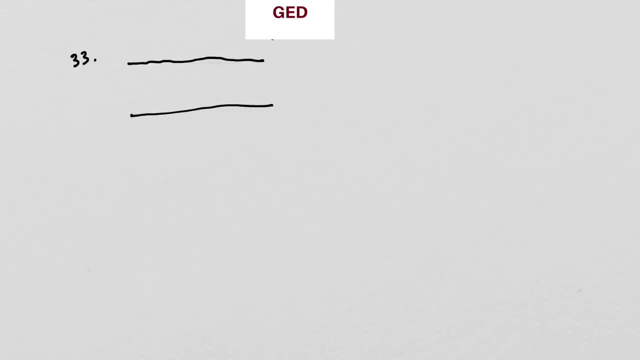 the problems that we see at typical GED questions, to give you further explanation to other similar questions. okay, So today we are going to look at some questions that are. they kind of look hard, but you should be able to solve it so easily by learning from this video. Now we are starting. 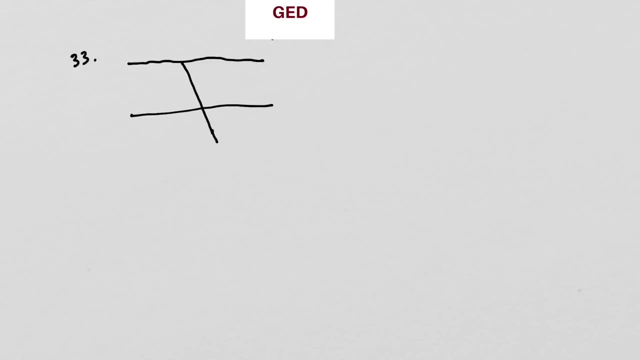 from number 33, because we have two previous videos. that covers number 1 to 32,. okay, Now we believe the best way to watch our videos or to follow what we are doing is to use the playlist which will be in the description, or I mean in a link somewhere. 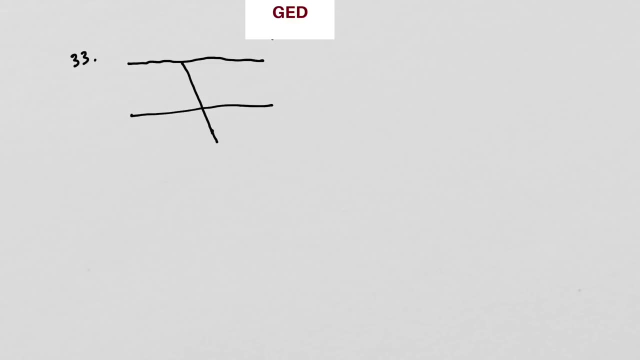 Okay, now, this is one question that usually comes in the GED. okay, So they tell you that this line and this line, they tell you they are parallel. okay, We use this dot to show that they are parallel. okay, And then they tell you that this is a transversal. okay, So a straight line, that is. 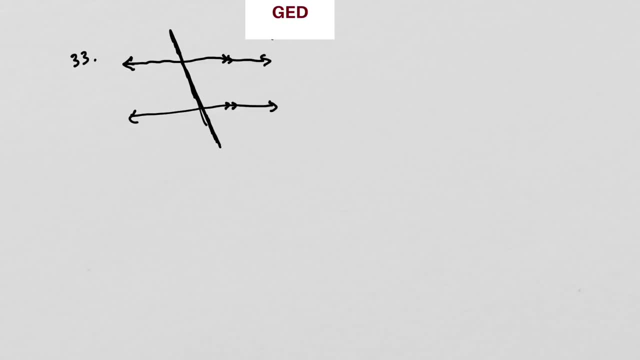 crossing the two lines And you are given a point. let's say this place is 30. This would not look like 30. Let me make it reasonable. Let's say this is 120.. Okay, and you are asked to find a bunch of things. So let's say you are supposed to find. let's say 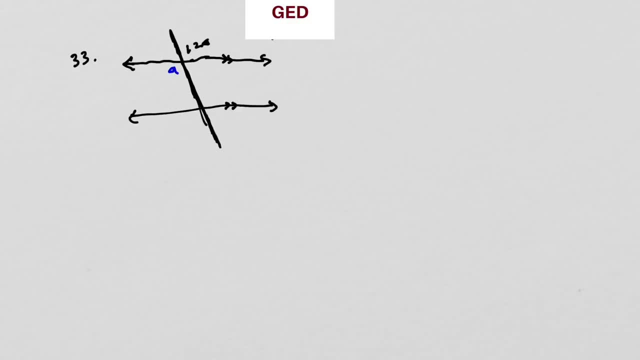 a Okay, so you are given the angle here to be 120. degrees, and you're supposed to find the angle a okay. now a few things. um, there are names for every one of these, but, uh, for this video we are not going to look at names. okay, we are just going. 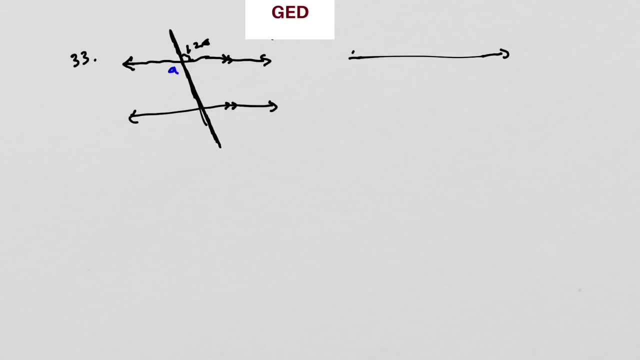 to look at how you can find all the angles that are available in a question like this. okay, so let's look at it. so again, we have our transversal. now the way i do this, i go about this, is: i label these things um. you can do it any how you want. i label this um. let's see a red. 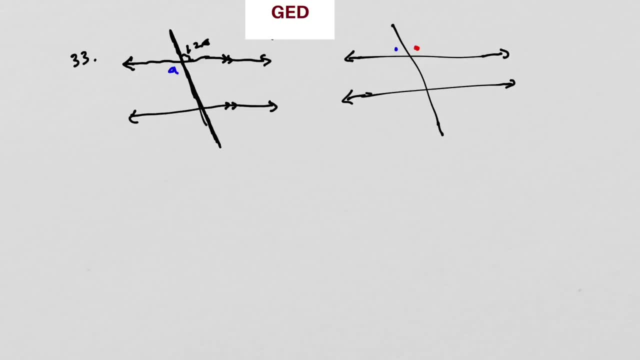 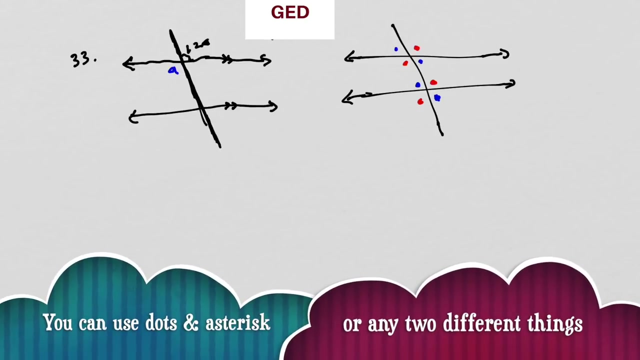 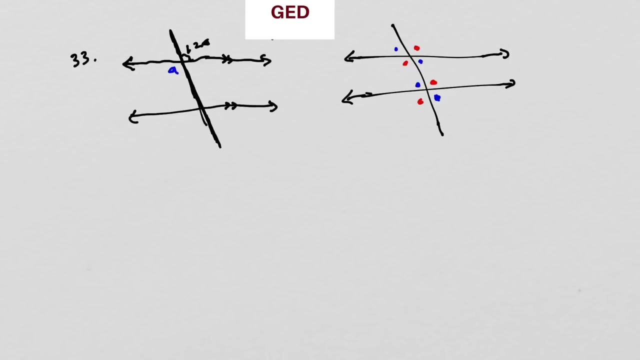 blue, red, blue, red, blue- i mean you can label it any how you, but you can see that we are just alternating. so red, blue, red, blue, blue, red, blue, red. it's just alternating. so you can clearly see now all the red colors. okay, so this is where every red color is the same as the next red color. 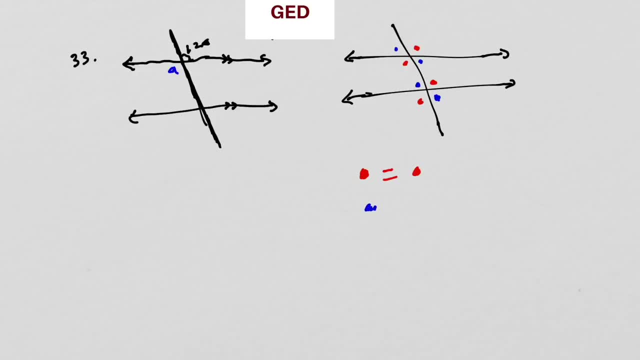 okay, every blue color is equal to the blue color, so the angle of every red is the same angle on the other red. the angle of every blue is the same as the angle blue, and the last thing is an angle on the red plus an angle on the blue will give you equals 180.. so that's all you need to solve. 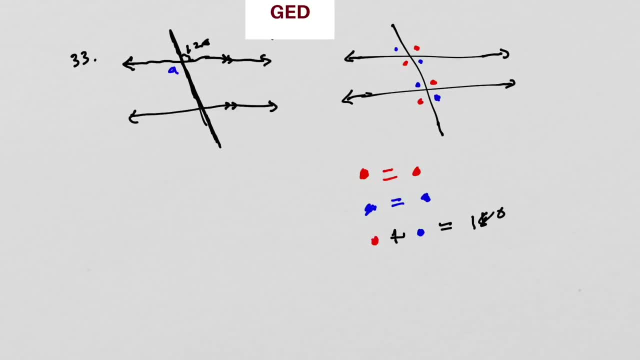 problems here. okay, so let's look at here. okay, so, assuming you're given that um this place before we come to our actual question, okay, let's, let's actually do our question. it says that this place is 120, right, so if this place is 120, that means all the places that you see the color red will. 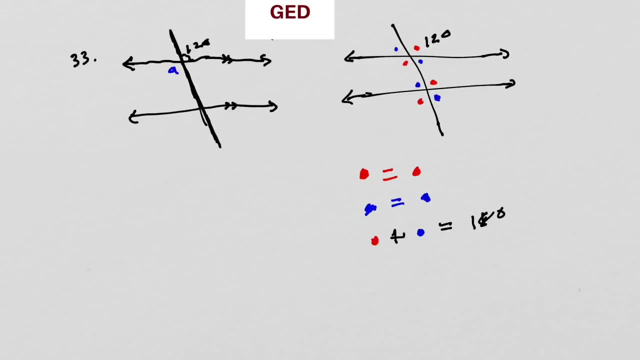 also be 120.. so if this place is 120, which was this side, then a, which is also red, will also be 120. so a equals 120.. okay, so it's as simple as that. so now we said, let's say we want to find. 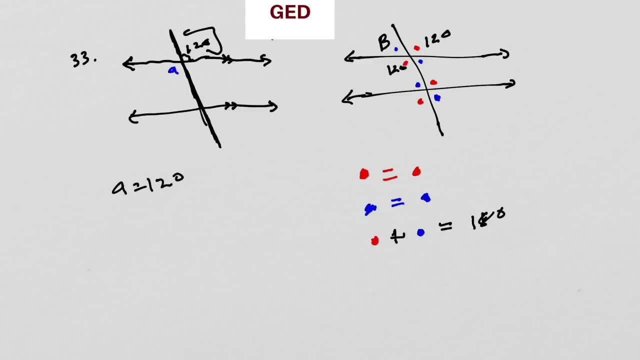 let's say this is b. okay, we want to find the angle of b. now, how do we find the angle? we said when you add a red and a blue, you get 180. okay, so that means red is what? 120 plus the blue, which we don't know. 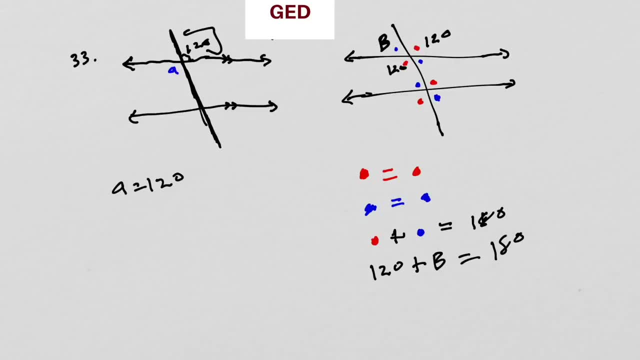 it's b equals 180.. okay, so to solve it, um, we just subtract 120 from both sides, so this will cancel out. so d will be equal to 60 degrees. so this is pretty much it. i mean, there's nothing difficult here, so let's just. 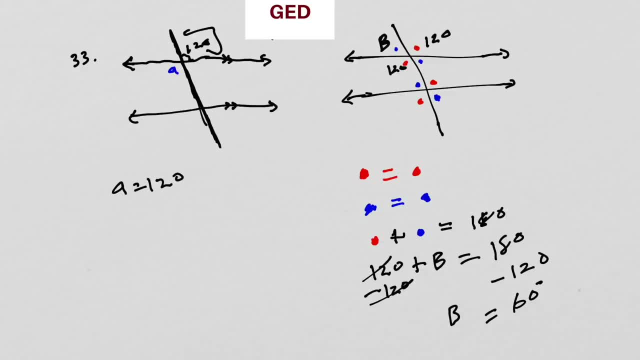 let's just try another question from you. okay, let's call number 34 again. i'm gonna quickly bring my um diagram thing here. i mean the transversal can fit into that can face anywhere. let me draw the transversal here, okay. okay again, I'm. 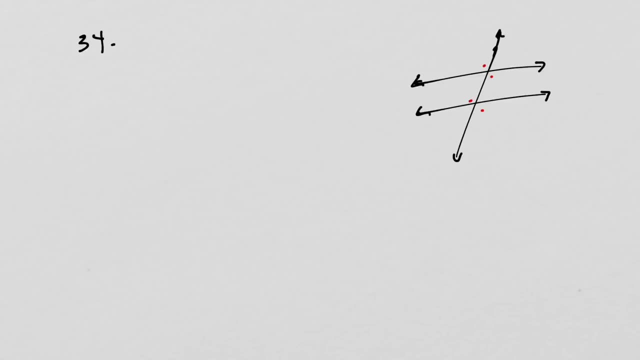 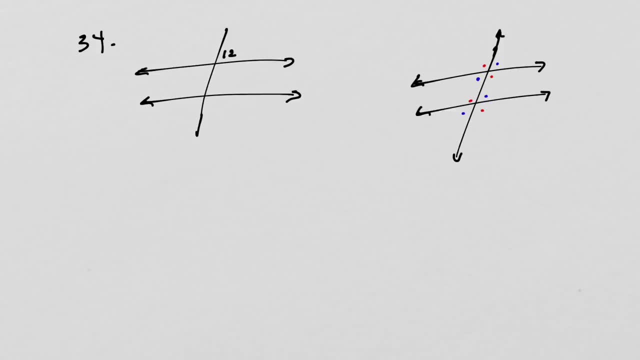 don't know, I like I'm doing things. but let's say we've been given this place to be 80, you've been given this place to be 80 and you're asked to find let's say this is X, okay, so again, straight up, you know. 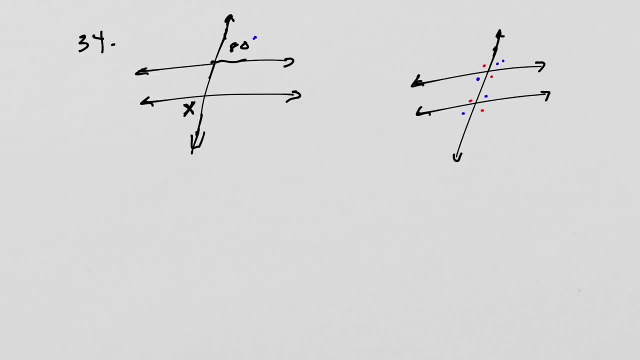 that this side is blue, okay, and then this side is also blue, right. so straight up you can say so easy: man X equals 80. there's nothing I mean strange or difficult about it. I mean they are here, your names for this. alternate angles and opposite, equal and radically episode. 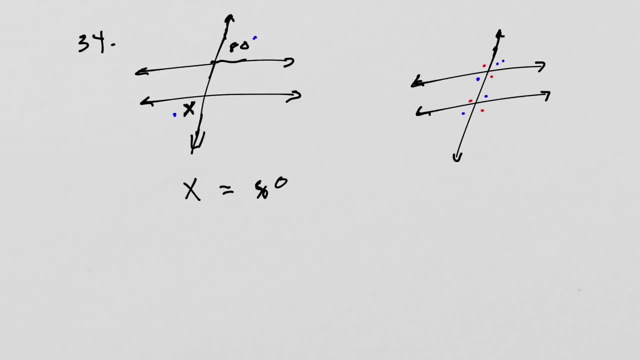 angles and all those. but you really don't need those things to solve. so let's assume now you are supposed to find what I'd you want to find. let's say you want to find this right. let's say this is m. so now said x is 80, right, so x and m must be equal to 180, right? 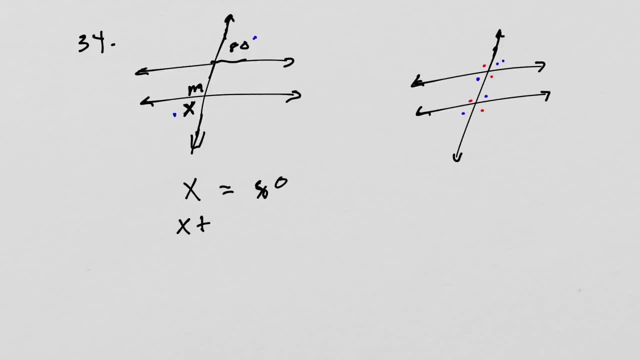 okay, so we know that x plus m equals 180. okay, so we know x is um. x was 80 plus m would be equal to 180. okay, so to solve this, we just subtract 80 from both sides, so this will cross out this, so m will subtract to get 100. 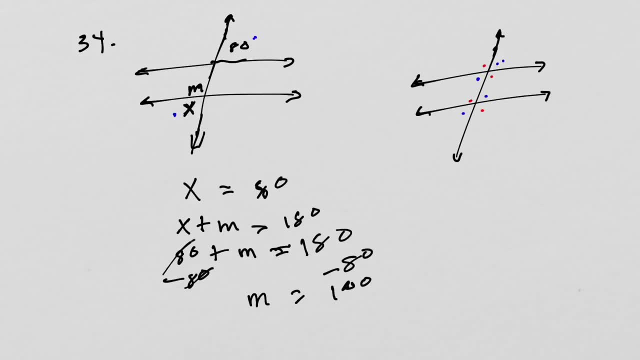 okay, so this is pretty much what this is. okay, so we are going to move on. let's erase everything here, okay. now another kind of simple question that comes in geometry especially. let's say, this is 35, um, it's questions that have to do with triangles. okay, so this is my triangle, okay. 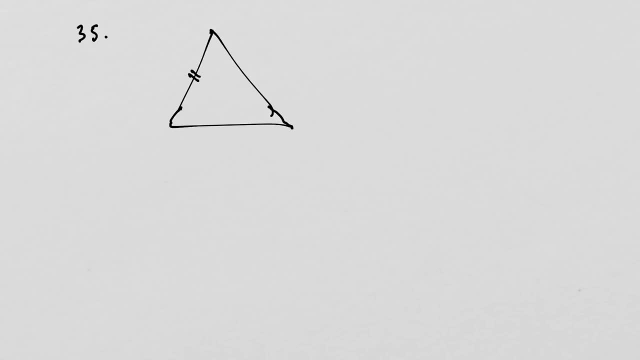 the first thing that we are being told about this triangle that this side and this side are equal. okay, now, all the angles in a triangle are up to 180. so this is: let's, if you call this a, b and then c, then a plus b plus c will be equal to 180. 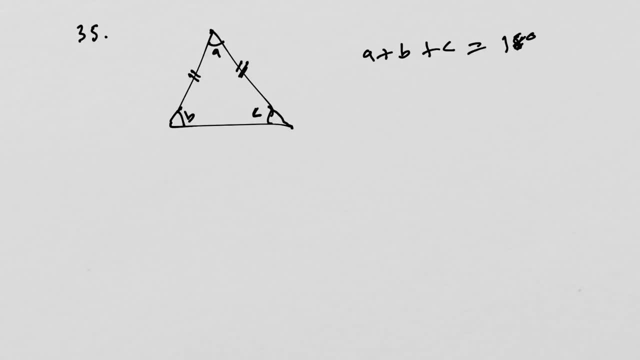 degrees. okay, so to we've learned two things right now. so okay, now this: we are told that this side and this side are equal. okay, that means it's an isosceles triangle and it means that the angle here and the angle here will also be the same. okay, so if b is, let's say, um 40 degrees, 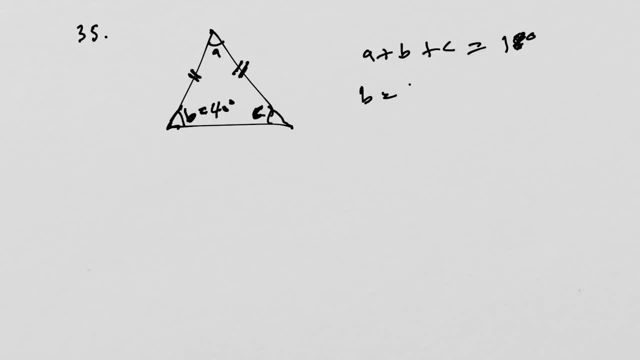 then c will also be. so b equals 40, then c will also be 40. okay, so, if you want to find a, then it will be a plus 40 plus 40 will be equal to 180. okay, okay, so we have. we add this two to get a. 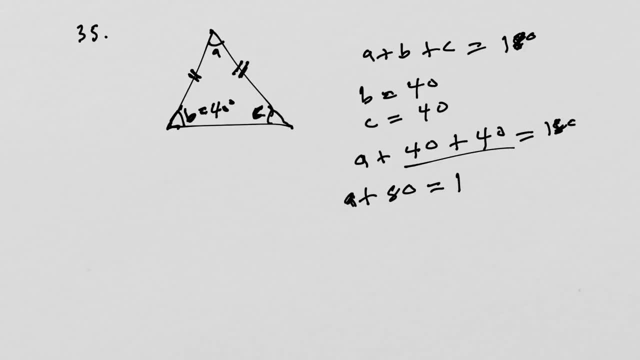 plus 80.. okay, so we have. we add this to to be a plus 80.. equals 180 again. we just subtract the 80 from both sides. this will cancel out this to get a equals um 100. okay, so let's look at more geometry questions. 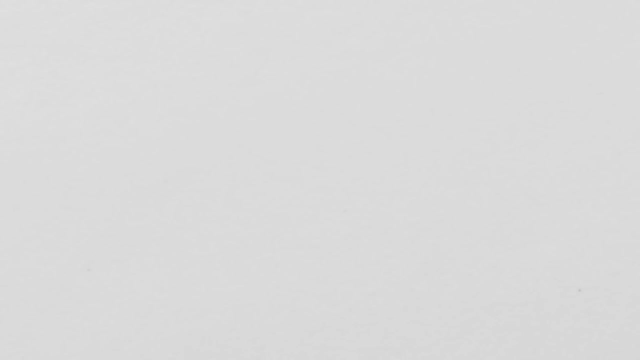 these are very simple. let's look at another one. this is another kind of geometry question that comes. so you are given a triangle this way, and then you are given a line that crosses the triangle and you are told that this line is parallel to this line. okay, so you are parallel. 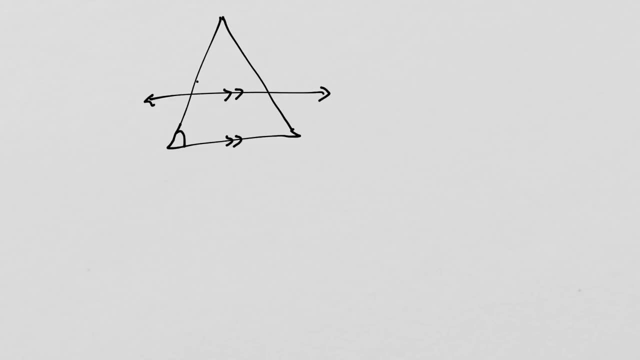 okay, so that means this angle will be the same as this angle, and this angle- let me use red- will be the same as this angle. okay, so if this angle is 50 degrees, then this will also be 50. okay, so if this is- um, let's say- 60, then this will also be 60.. 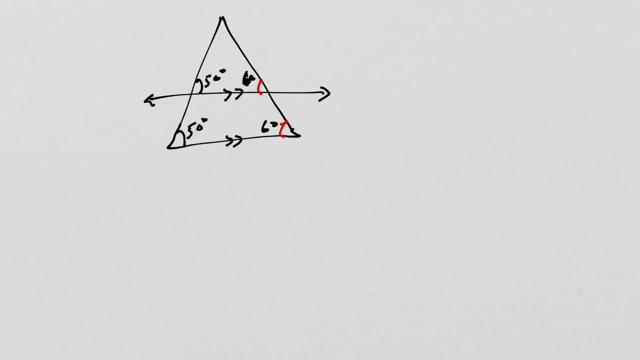 okay, so that's this also very simple. um, okay, now we're moving on. let me erase this. so let's go to number 36. okay, now for 36 we want to look at- uh, we are moving away from the geometry questions- and for 36 we want to look at something that is also very simple, but i mean students, some. 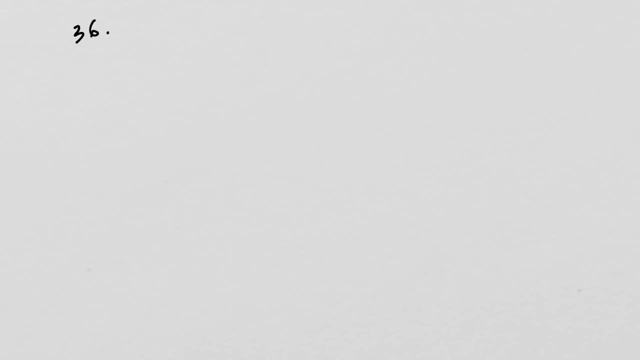 students do get it wrong. now, let's finding a fraction from percentages. okay. so let's say you have 20 percent now to solve um this. say, change it to um fraction, okay, okay. so all you do when you see a percentage is 25% a percentage, it means it's over 100. okay, so this is simply 20 over 100. okay, you saw that the first. 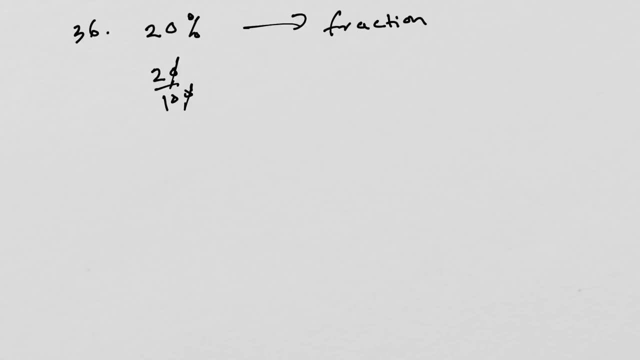 thing: if you see zeros, you can cancel out the zeros. so now you have to reduce 2 and 10. okay, 2 can divide 2 to get um 1, and then 2 can divide 10 to get 5. so this will be your fraction answer. 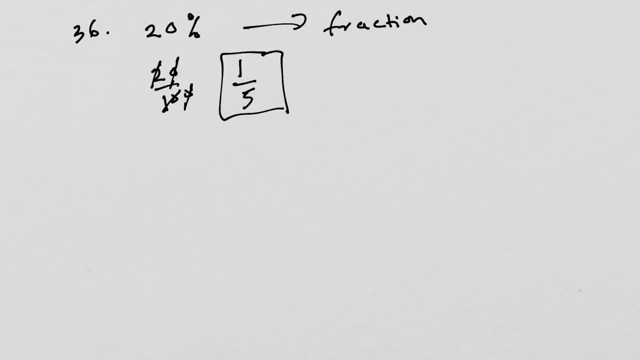 okay. now to even convert um percentage, let's say 20, i mean 37. to convert percentages to um decimal, it's even easier. okay, you're just moving the decimal point. okay, so 20 um percent to decimal. okay, okay. so 20 percent is the same as 20 over 100. okay, 20 over 100. 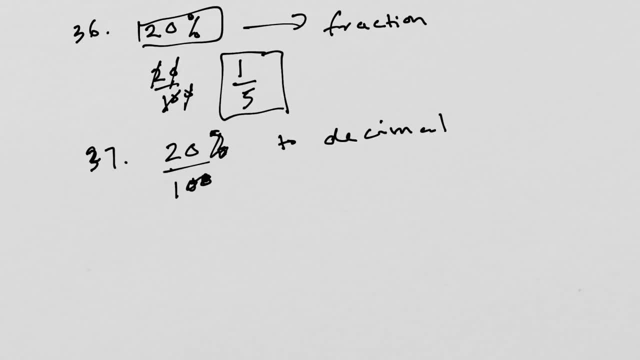 we know that already. so this zero is just this. two zeros is just going to move the um decimal point to. we assume that when you have the whole number, let's say 20, there's a decimal behind it. okay, so if you see any number, let's say 70, without any decimal point. the assumption: 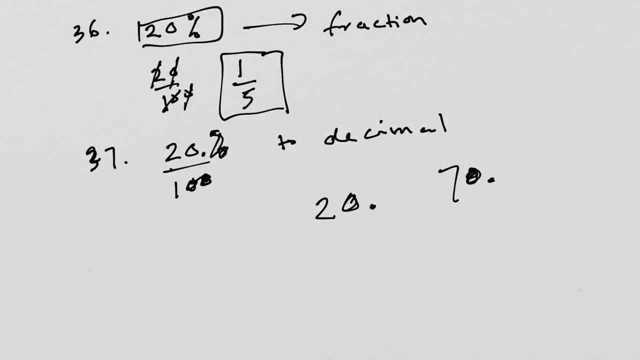 is that there's a decimal points behind it. okay, so if you're supposed to um find, i mean change the decimal, then you're just moving it two times to the um, to the left. okay, so one, two. so now you have 0.70. there's no need to write this zero, you can just write 0.7. 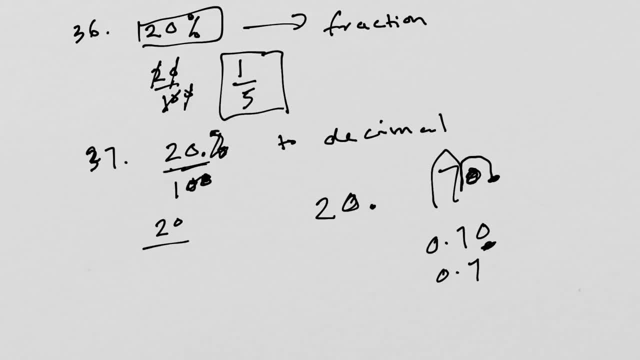 okay, so now let's come to our question itself. so here we have 20 over 100, so we said there's a decimal assumed decimal at the back, so we are moving it. two zeros to the left, one, two. so we have 0.20 and we said that zero is not important, so it's simply 2.0. okay, let's look at the 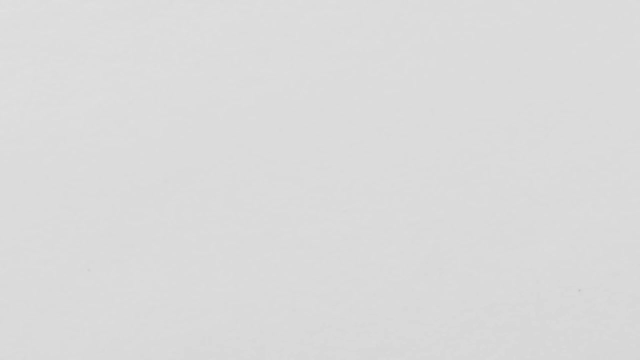 add it again. okay, um, now, finally, um, this is just a practice, so for those of you just want to keep on watching the rest of the video, uh, we just want to go through some other basic things. i mean, it's not really part of the question. one of the things that we have noticed that a lot of students get wrong. 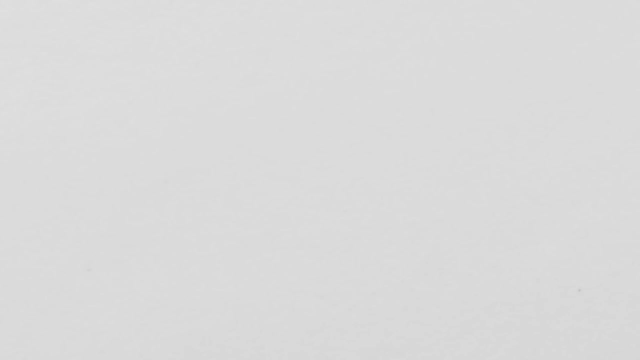 um, are working with um negatives. okay, just simple addition and subtraction of negatives. okay, so if you're familiar with it, you can actually skip this part of the video. if not, you can just join us. so that's what we are going to do right now. okay, so let's look at this question. 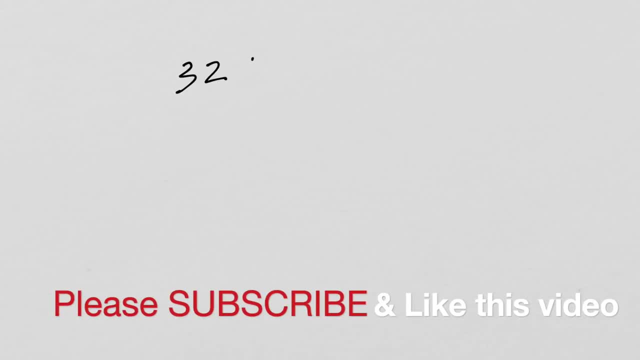 so let's say you have 32 um plus negative three um, and then let's say 32 minus negative three. so here, what we are supposed to be putting in here is whether it's less than, greater than or equal to. okay, so we are supposed to solve this. 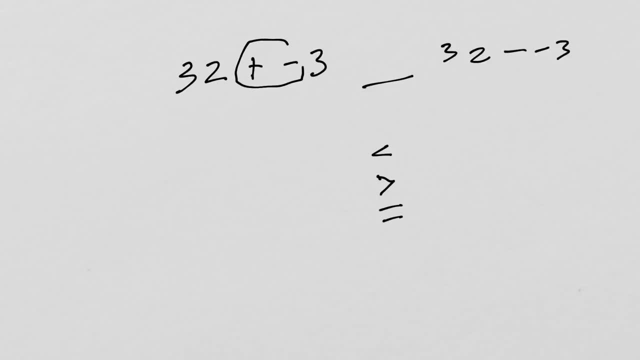 question: okay, so now this confuses a lot of students, okay, okay. so when you have a minus negative, it becomes a plus, okay, and then when you have a plus negative is the same as minus, okay, okay. so here we have 32 minus three, dash, 32 plus three, okay, so obviously we can see that this will be less than that, okay.